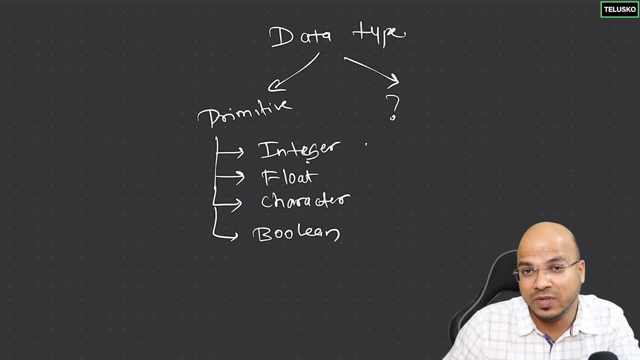 you go with characters like a, b or any regional characters you have all across the world. that goes into character. and then, when it comes to true and false, we go with boolean. Now, inside integer itself, we have multiple subtypes to it, We have a concept of byte, we have short, we have int. 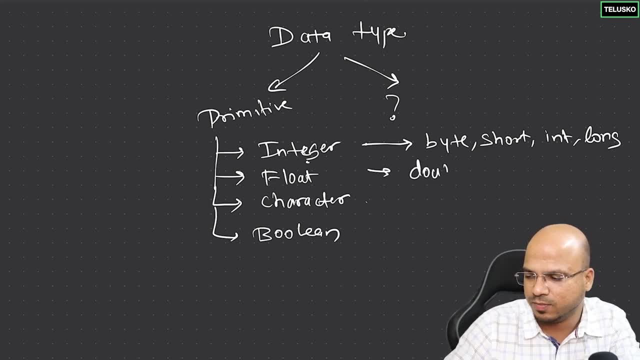 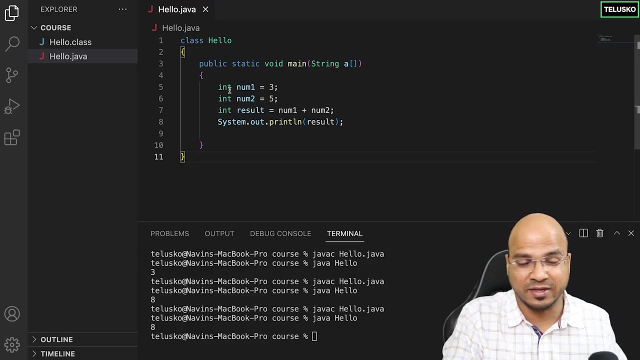 and we have long For float. we have another option, which is of double, and then of course, we have float and then characters are characters. So in characters we can have different type of characters. In boolean, the only values we can have is true and false. okay, So, example, if I go back to my code and if I want to create a different variable this time, 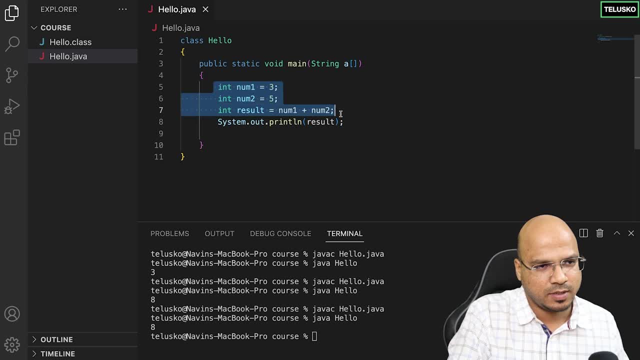 let's say float. So I can just come back here, I can remove this section and here I can say this: we are creating a float value. Now, how do we get a float value? So we can simply say float and then we can have a value. let's say seven, or we named it right. 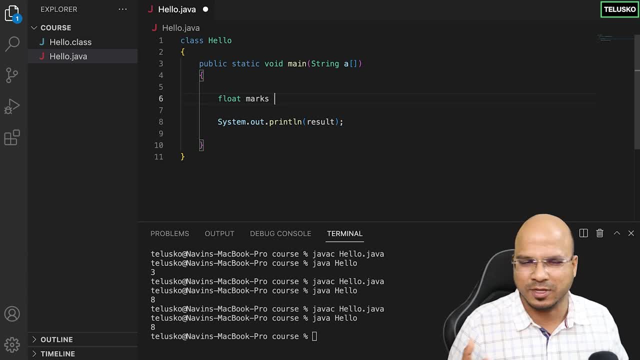 So name we can have is marks. of course we don't put in marks, but let's go with now marks. and then we can go with a value. Now, floating by values will be having a dot, right, so we can say 6.5, something like this: So float marks equal to 6.5. that makes sense, right? Okay, cool. 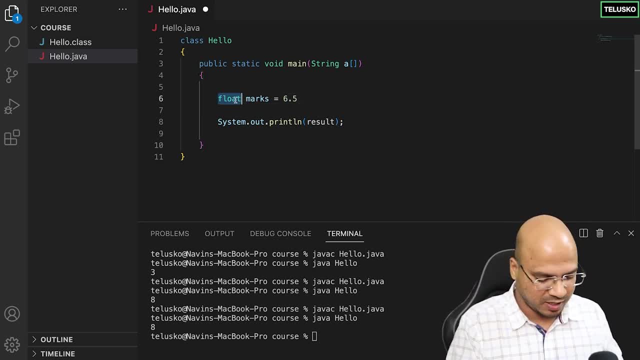 In the same way, we have also mentioned, we have subtypes to integer. we can have a byte format, but why do we need all these extra formats For that? let's understand some basic concept Now about integers itself. so if we talk about integer, we have some sections to it, so integer will have 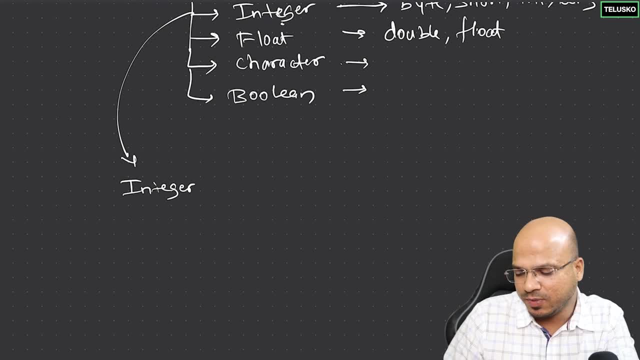 different part, So integer will have different sizes, Example if you want to store a normal number. so in general we always go with int and int has its own value. Okay, so when you talk about int, the size of int is is four bytes, so we can say 32 bits and then it has a range to it and you can. 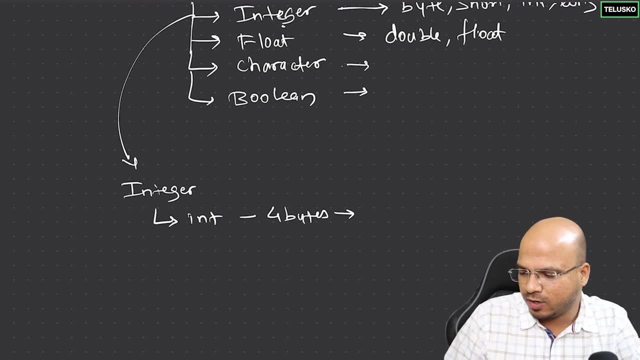 find the range on the screen. We also have a format which is, let's say, if you want to store a bigger value, a very big value, So in this case, and of course the value goes beyond that range, we have to go for a long format Now. long supports eight bytes. Now, of course, when you have more bytes, it. 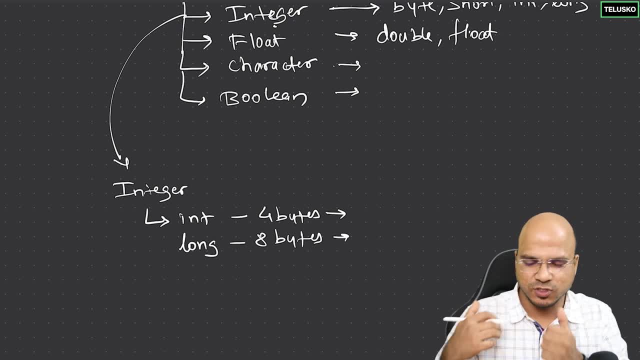 will. it will occupy more values and it will have a range. so of course you can find the range on the screen. Now what if you want to store a smaller number? so of course int provides you the range. but then what if you want to save memory? you don't want to go for int range? In that case we can have 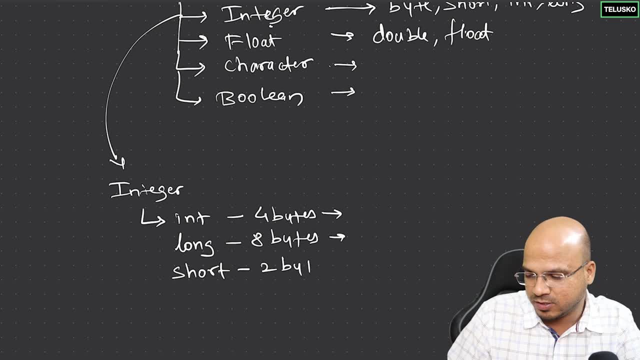 a short value. Now, short is only two bytes. So if you want to have a limited range, you can find the range on the screen, and then we have the next range, which is of byte. Now, byte is only one byte. Okay, so eight bits and whatever you want. 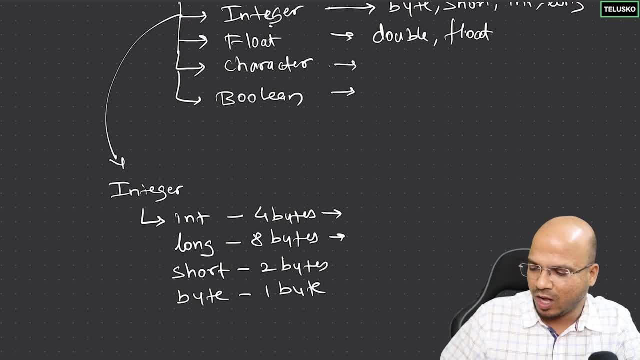 to store. you can store in that, Of course, it has its own range. Now how do we calculate this range? So we do with the help of it goes from negative values. right, so it is minus two raised to eight. two plus two raised to eight minus one. Okay, so which is two raised to eight, is what it is. oh, we're. 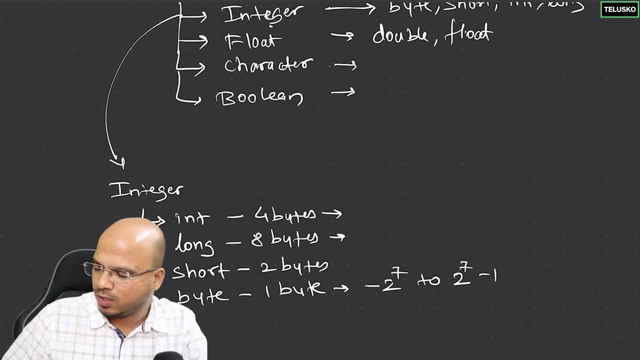 doing right. so it is two raised to seven and two raised to seven and the range it's. so how do we calculate? two raised to seven is 128, so it starts from minus 128 to plus 127. so 128 minus one, 127.. That's how you can calculate the range for all the other numbers, and you can, of course you have seen. 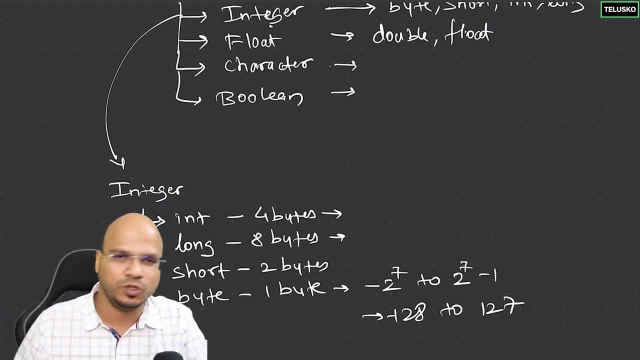 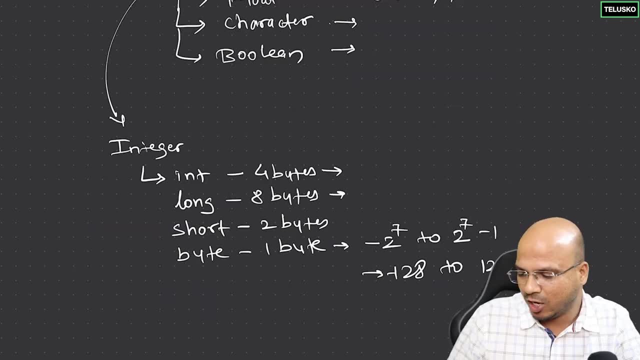 that on the screen. So this is how we can use integer. so which one to use. so if you want to get a variable which is a, which will have a value, let's say five or six, or maximum 127, you can go for byte. Now how do we get that variable? It's very simple. you use a type which is byte. you use: 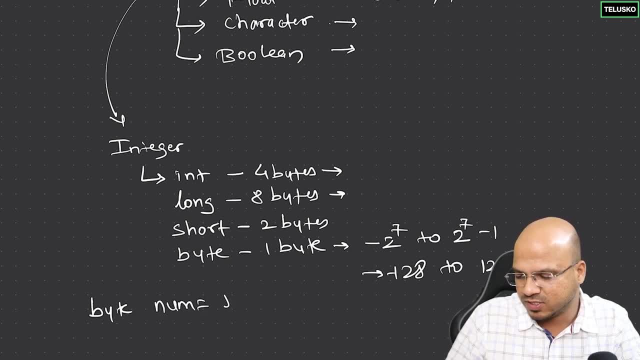 specify a variable name, let's say num, and you assign a value which is eight or any other value which you want. Of course, that should be in a range and that's how you can store it. Now, what if you want to have a float value? Now, float actually gives you two different values, or two? 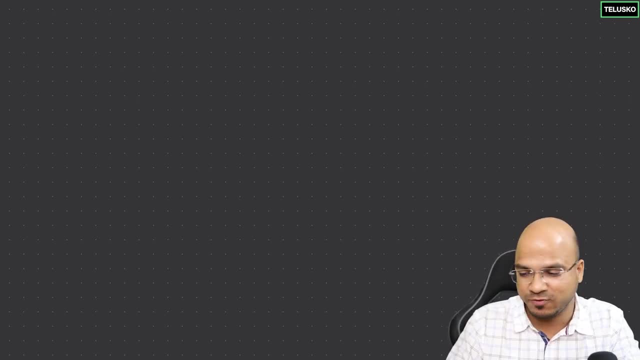 different types. Now it depends upon which programming language you have worked with before. Example, if you have ever worked with C, by default we have a value which is float, So by default we have float there. Now float only takes four bytes and it has its own values you can store and then 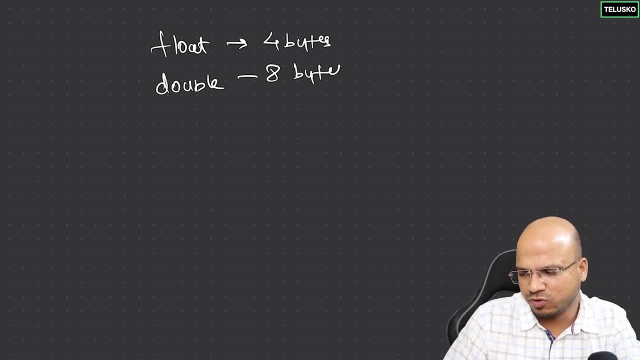 double, which takes eight bytes. Now what do you think which will be default value? Think about it. will it be float or double? by default in java. So default is actually double, not float. okay, Now, why double? is because, see, float are good when you have limited values, when you have limited precision. 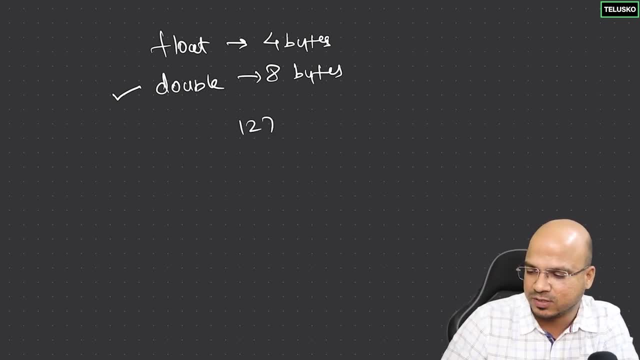 because after your point value, example, if you have value which is 126.5678 or whatever values you have, so float will have a limited precision set here. but on the other hand, double will have a longer one right, So double will have a longer one right. So double will have a longer one right. So 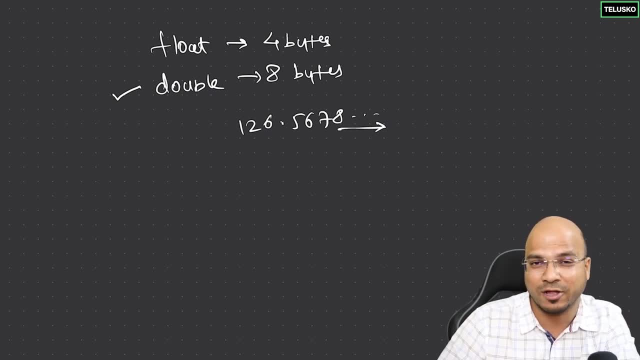 double can have more values. So whenever you perform scientific calculations or any kind of calculation, if you wanted to make it fast and it would support maximum precision, you can use double there. right, and by default, java supports double. So if you want to create a variable which is with 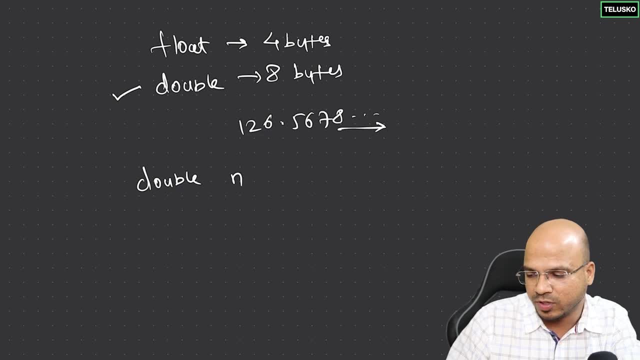 double. so you can simply say double and you can create a variable. name: num is equal to. you can assign a value which is 5.6 or whatever value you want to assign. But how about float? Now, if you try that with float, it will. it may not work. Example: if you say float and if you say a variable. 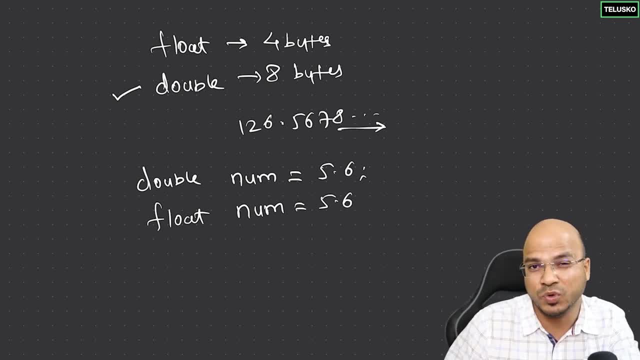 so when you try to assign 5.6, it will give you error. it's because, by default, the moment you say point values, it will be considered as as double. and if you want to say, hey, i don't want to work with double, i want to work with float, so explicitly you have to mention, hey, okay, this is actually double. 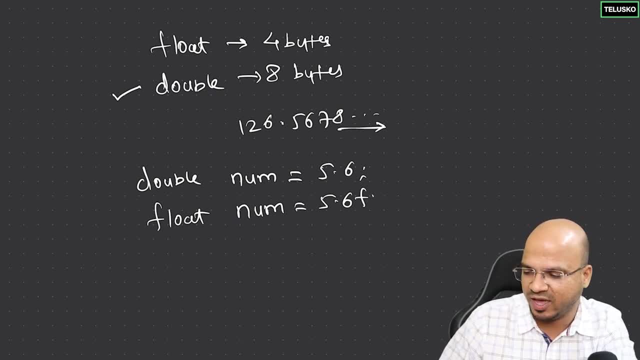 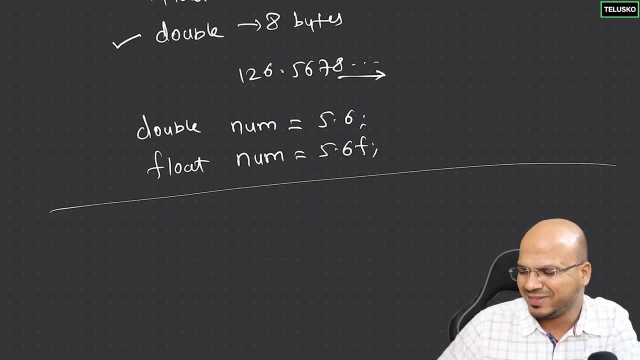 value, so you can. this is actually a float value, so you can put a f there, right? so 5.6 f, that's how you define. it's a float value for double. you don't have to mention that now. how about character? so in other languages character will have a less bits, but in java it goes for two bytes, so in 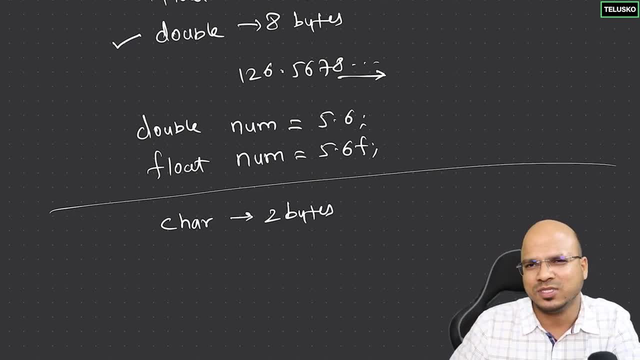 other languages, like c, you have only one byte. it's because it normally occupies the integer range. it normally occupies the character range, ascii values. but then in java we thought, hey, can we just have all the characters in the world, not just english, all the languages. so java actually follows. 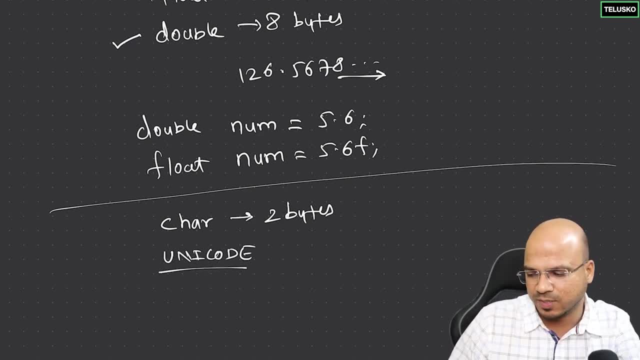 something called unicode, not ascii. by default, it will support unicode and it has two bytes, which is 16 bits, and that's why it's called ascii by default, and it has two bytes, which is 16 bits, so it has a bigger range, right? so this is a range it normally works with, so of course, you can work. 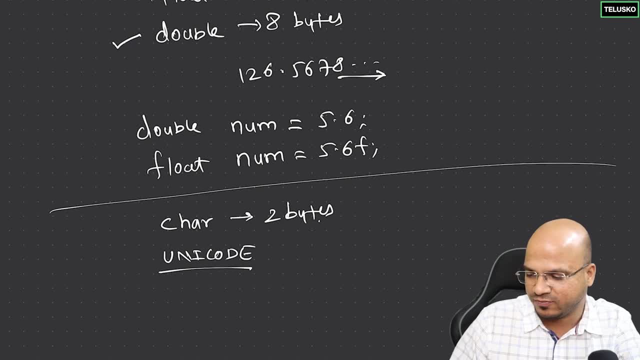 with any type of values you have and any type of characters. basically you have- and if you want to define a character variable, it's very simple. you say char and then you specify the variable name. let's say character or c, equal to whatever character you want to assign. let's say i want to. 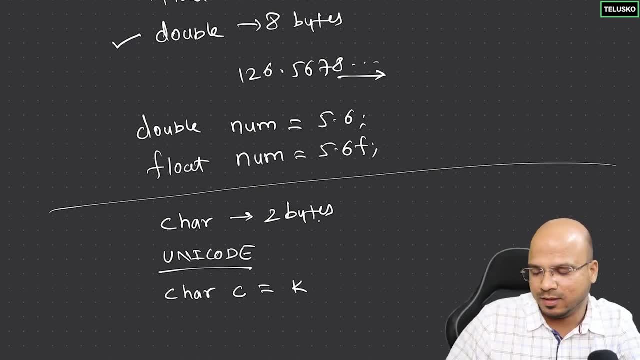 assign a character which is k now in this k. in this case, if you want to work with a character, can we use double quotes? now, double quotes is for string, right for character. we have to use single quote and you have to put your character into single quote and you have to put your character. 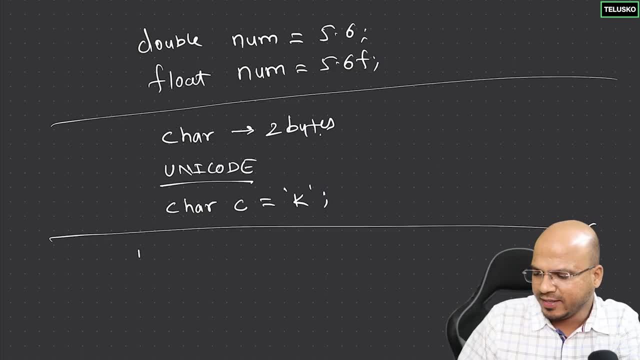 into single quote and remember it will only accept a single character. and next we have of type boolean. so if you want to work with boolean now, boolean will only accept true or false. okay, no other. there's no subtypes here, only true or false. now one thing you have to remember now, in other 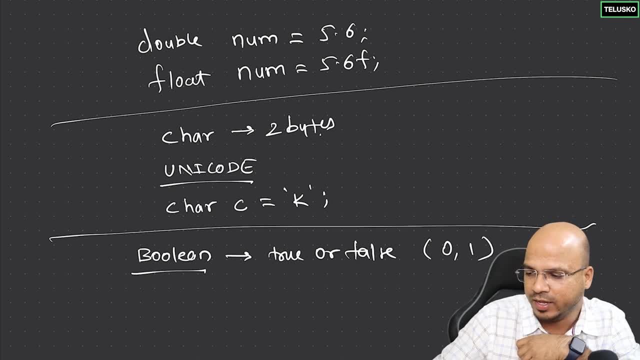 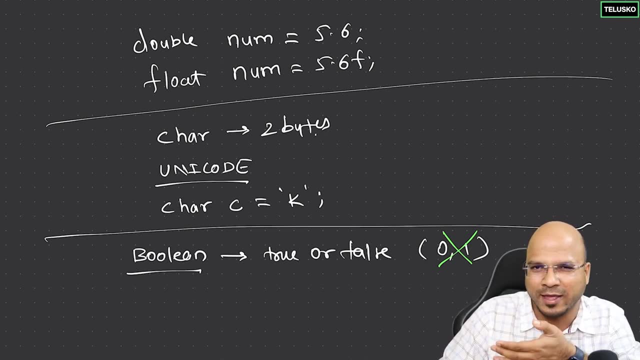 languages. it may represent it with the help of one and zero. in java we don't do that, so in java it does not. it doesn't work with zero and one. it is true and false. there's not like true is one and false is zero. it's only true and false. 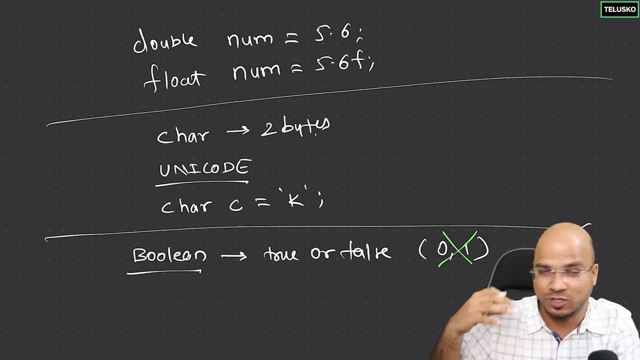 it is normally used for conditions. if you are want to check for a condition based on that, you will do something. that's why we can use true and false. i mean think about computers. when you say computer can think, it's because of this true or false. okay, and how do we define a boolean variable? 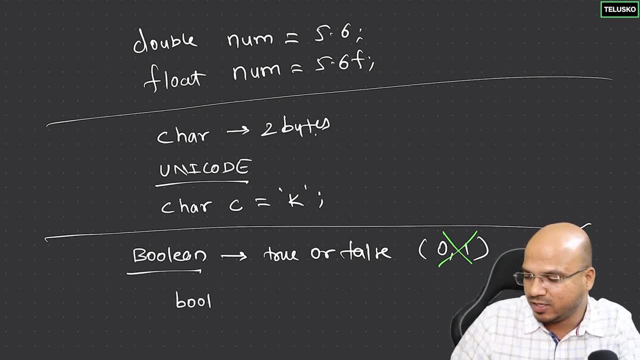 so it's very simple. you use a keyword called bull and then you mention a variable name. let's say b is equal to. you either assign true or false. okay, you don't have to put a single quote or double quote, because they are itself keywords. so these are the options we have now, if you want to see. 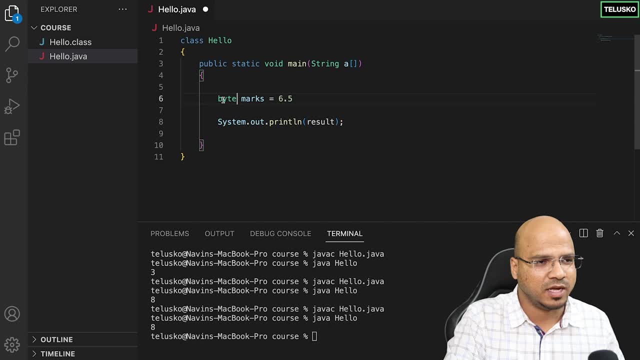 very simple. you can just go back here and say, okay, byte is done, let's create some variables with different type. so int we have already seen, so it's a num one. this is how you assign integer value. but if you want to go with a byte, so you can say byte b or we'll say by equal to now can. 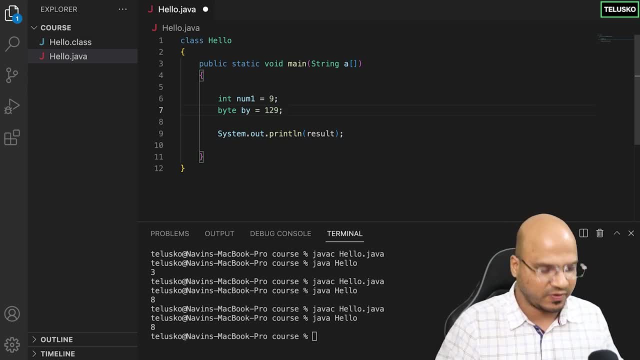 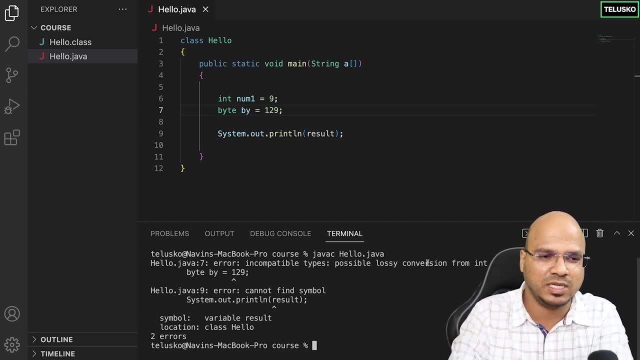 i assign a value which is 129, you can see it will give you. if i do that, if i go back to my compiler compile, you can see it will give you error. it says possible lossy conversion from into byte. so this is which is 129: it will. if you try to save that in a byte will not work. but what if you say 127? that's. 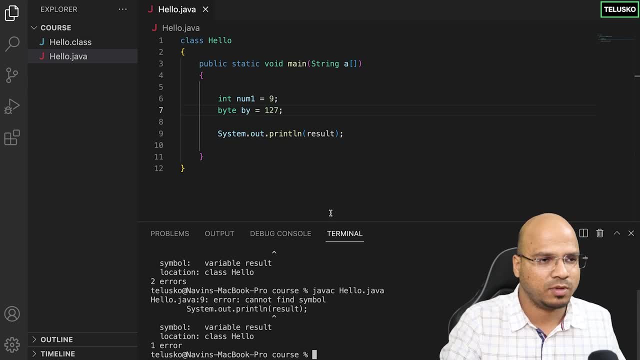 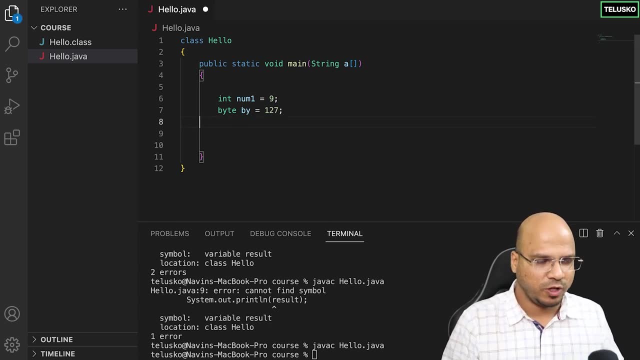 the last value you can store: compile- okay, there is a problem with result. let me just remove this section and compile. no issue, okay. so this is how you save byte value. what if you want to store short, so you can say short, sh equal to and you can assign value which is, let's say, five, five, eight. 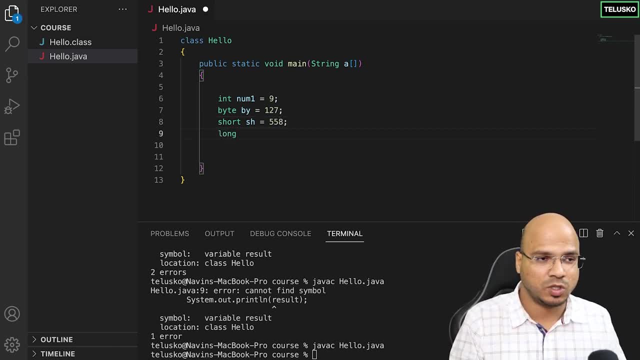 any number doesn't matter. and then what if you want to work with long, so long equal to now? when you work with long, remember this thing: after every number for long, you have to put a l at the end to specify that's a long number. the thing we have done with float, we have to put 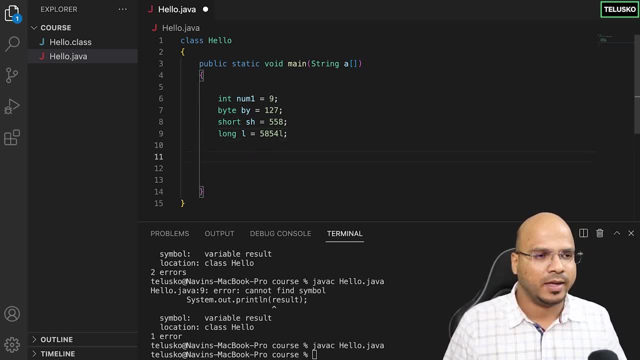 f in the same way, long needs l. and what if you can do here with float so you can say float f is equal to 5.8? okay, let's try with 5.8 and let's see what happens if you try to compile this. compile okay. 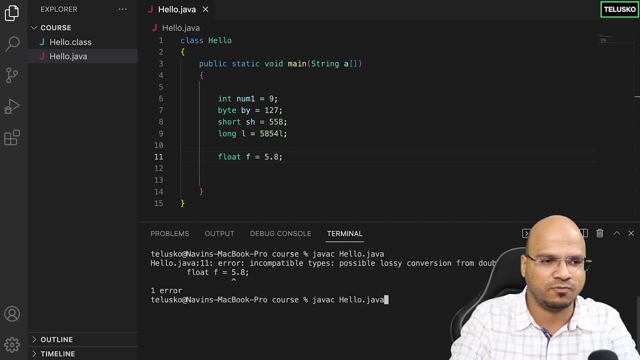 you can see it is giving you error. it says again: possible lossy conversion from double to float because by default 5.8 is double. if you want to mention, hey, that's not double, that's float, you can put a f at the end. that should work. you can work with double as well. 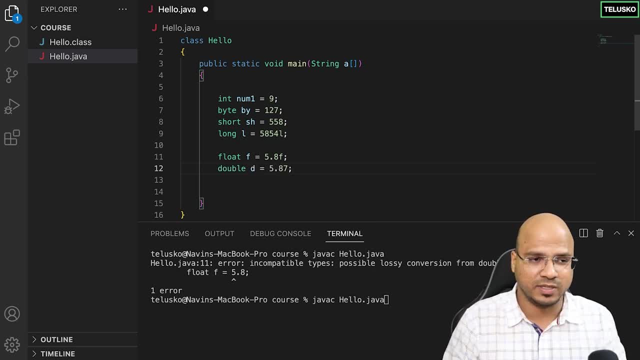 double d is equal to 5.8. same value, but this time it is double. and then what else we can work with? we can work with character as well. so we can say: char c is equal to. in single quote you can mention a character k, then we can go for boolean, which is boolean in this case, and you can say: b is equal to. 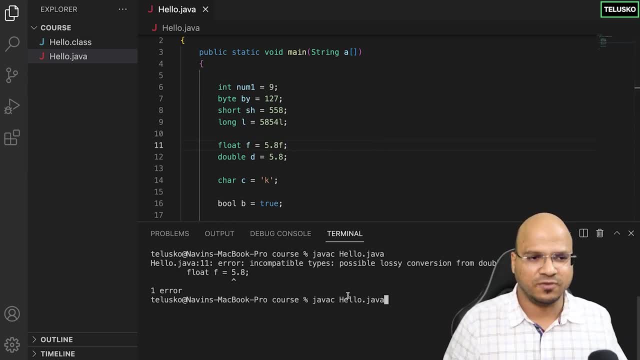 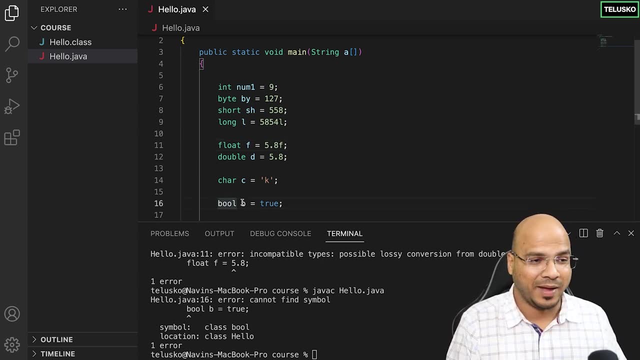 true, simple stuff, right? uh, let's try to compile this. of course we are not printing anything, so you don't expect anything on the console compile, or there's an error. it says cannot find symbol bull. okay, my bad, it is boolean. the only problem is when you work with multiple languages at the same time, you get confused. 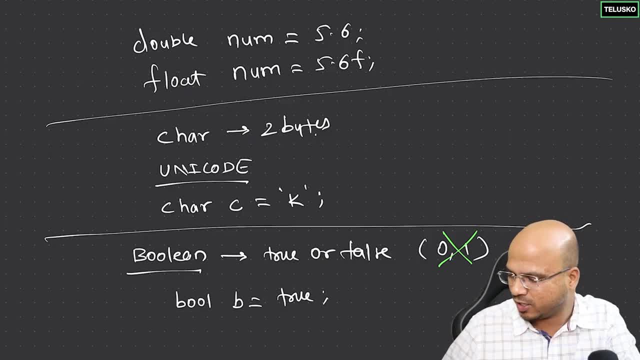 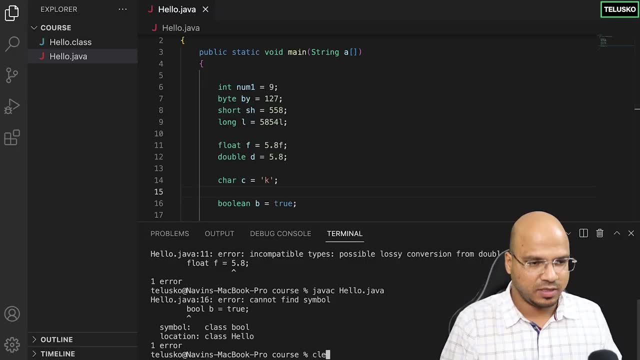 somewhere, so that that's boolean, not bull. so the nodes as well. i need to change it. so i will say: this is boolean, cool, and now let's compile this once again: compile, okay, there's no problem, and let's run this. of course it will run, but then you will. 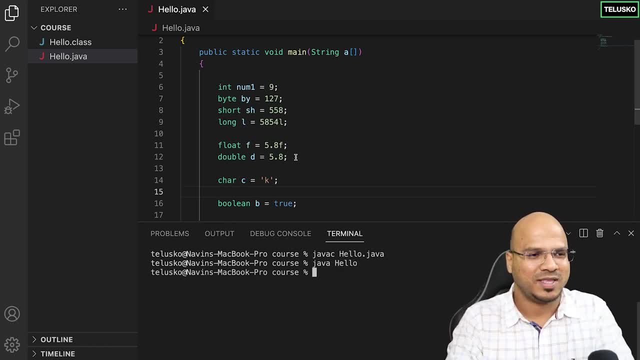 not see any output, right, no output, because we're not printing anything. so, yeah, that's about this. we have different type of uh data types we can work with, and all these are in build. apart from this, we also we also have some more data types which we'll see later. they're not type of primitive.